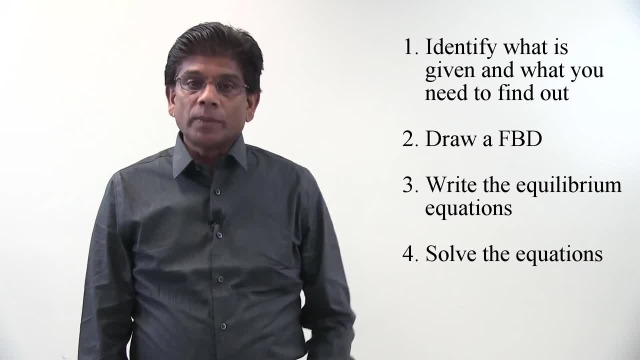 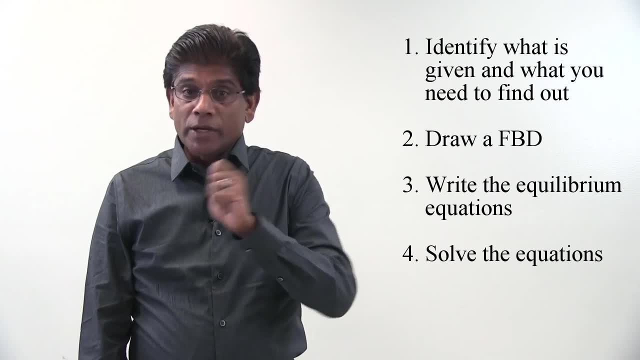 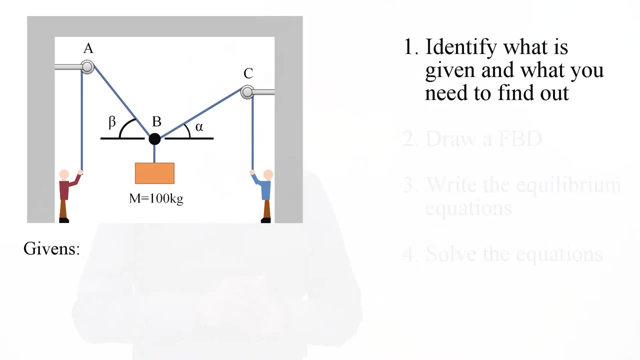 solve the equations using any approach that you are comfortable with To solve the equations of equilibrium. I highly recommend you learn how to use a calculator to solve the equations using a matrix approach. Let's now apply this approach to this particular problem. So in this problem you are 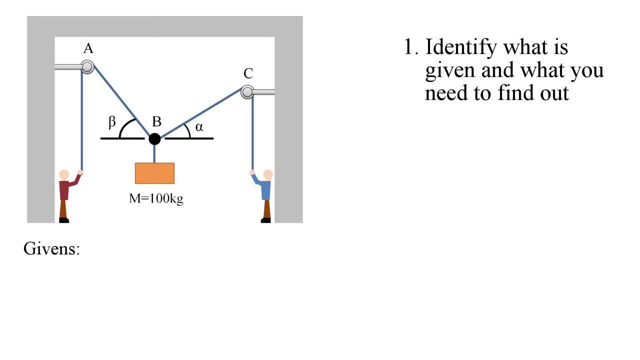 given the angles alpha and beta and the mass of the crate, Let's write this down: Alpha is equal to 30 degree and beta is equal to 45 degree. Since we want the weight of the crate and we are given the mass, we need to convert it. So let's convert the mass to weight by using the. 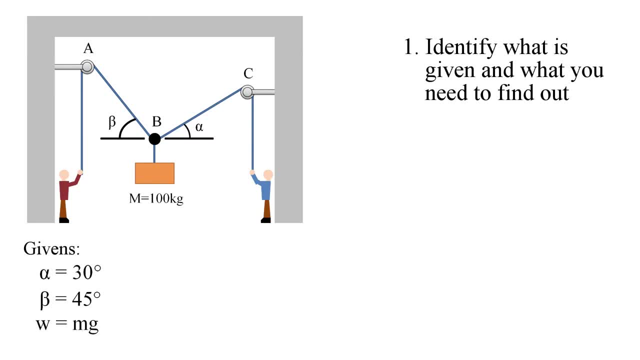 equation w is equal to mg. Now we need to identify what are the unknowns. In this case, there are two unknown forces. Let's denote these two forces on the cables as T sub AB and T sub BC. Now to solve. 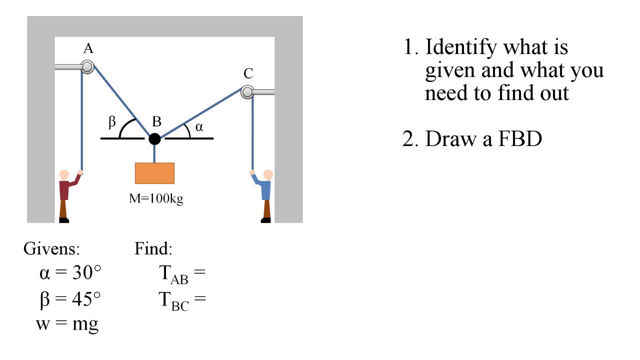 the equations of equilibrium. we need to use the equations of equilibrium. So let's take a closer look at drawing free body diagrams. first, I am going to use a step-by-step process to draw the free body diagrams. Step-by-step approach will make it easier for you to solve any problem with. 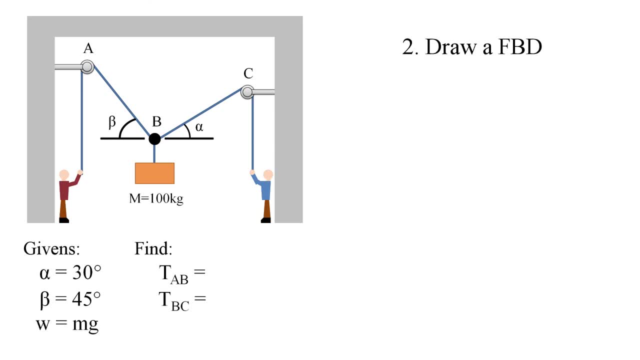 these In order to draw the free body diagram, isolate the body or area of interest. The crate is in equilibrium and if you look at the crate closely, you will realize there are three cables, and we need to. all we need to do is to draw the free body diagram containing these three. 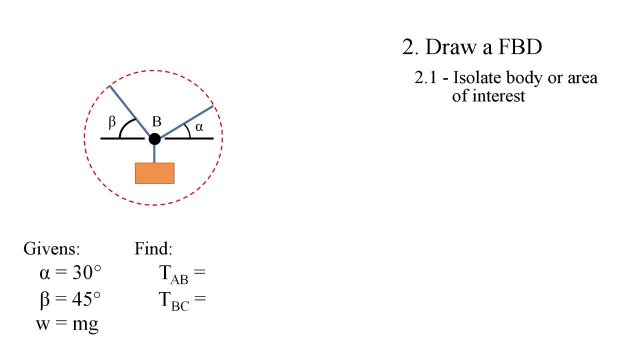 cables And these three cables are intersecting at point B and let's identify this area. Now draw an outline of the isolated part. This outline has got three lines coming out of point B. Each line has got three lines coming out of point B. Now let's show all the forces both known and 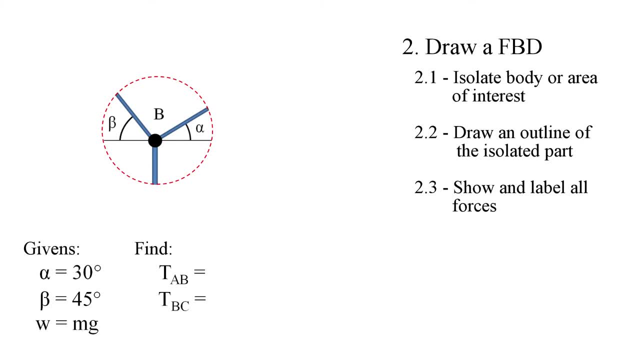 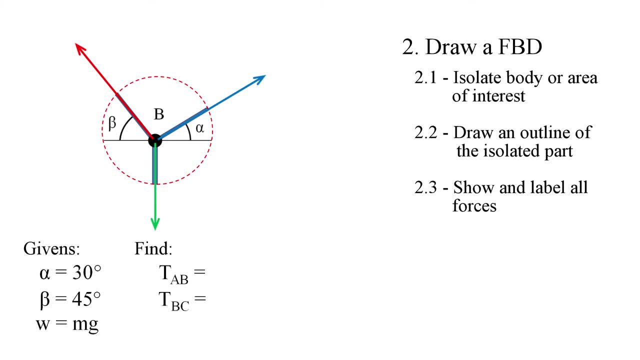 appropriate labels for the forces. In this case I'm going to write T sub AB for tension in cable AB, T sub BC, for tension in cable BC, and I'm going to write W for the weight. Weight is known and the two tensions are unknown. So here we have a diagram that shows all the forces. 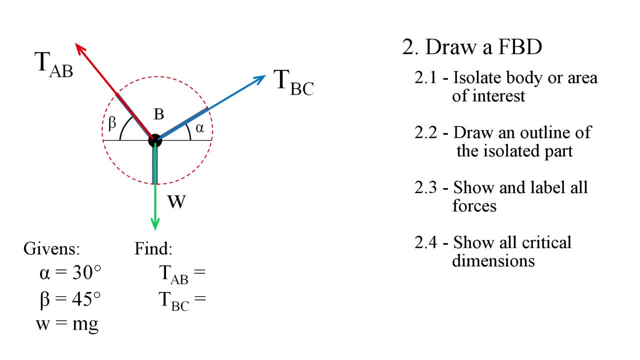 The next step is to show all the necessary dimensions. We need to write them down, So the critical dimensions in this case are the two angles, alpha and beta. Alpha is equal to 30 degree and beta is equal to 45 degree. Weight is 100 kilograms and we can convert that to force by: 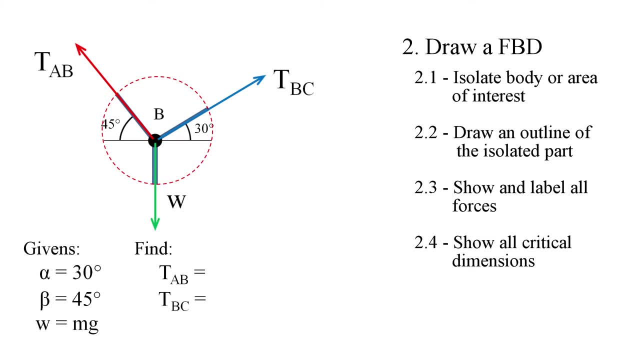 multiplying by G, which is 9.81, and therefore the weight is 981 Newtons. Finally, we always need an appropriate coordinate system to solve equilibrium problems. In this case, in this case, let us attach a rectangular X- Y coordinate system with its origin at point B. 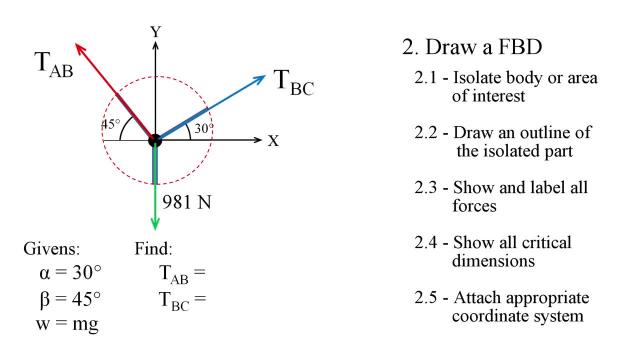 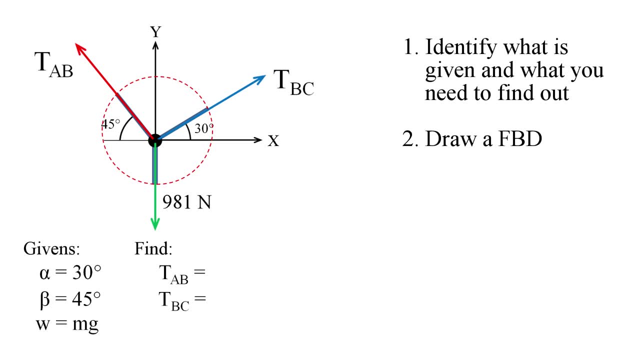 Please make sure you always draw a separate free body diagram. Do not ever draw a diagram right on top of the picture that is given to you. Now that your free body diagram is complete, we can write the equations and then solve. Let's write the equation. There is only 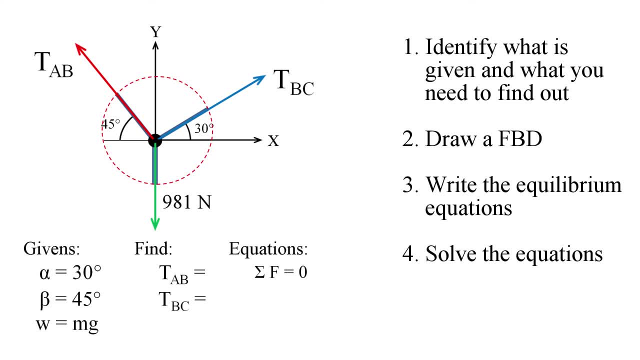 one equation: sum of all the forces equal to zero. This is a vector equation. We can rewrite this vector equation as two scalar equations for each axis. Let's sum up all the forces along x-axis. first, TAC times cosine 30 degree minus TAB times cosine 45 degree is equal to 0.. 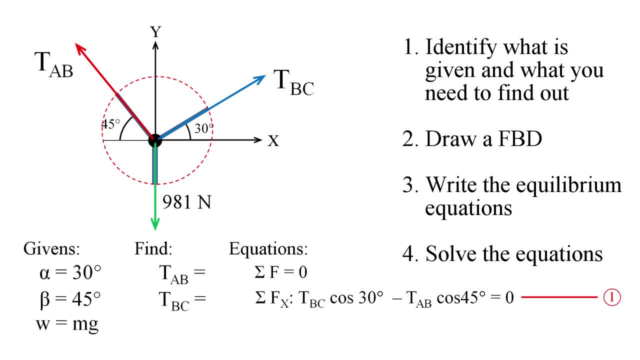 This is our first equation. Notice the negative sign for the force T sub AB, because the tension is in the other direction. Let's now sum up the forces along y-axis: TAC times sine 30 degree plus TAB times sine 45 degree minus 981 is equal to 0..